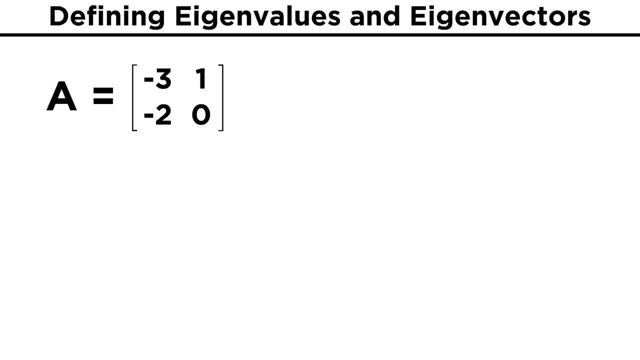 Let's say that matrix A is a two by two matrix with elements negative three, one negative two and zero. Now let's check that the vector x equals one. one is an eigenvector. Let's say that matrix A is a two by two matrix with elements negative three, one negative. 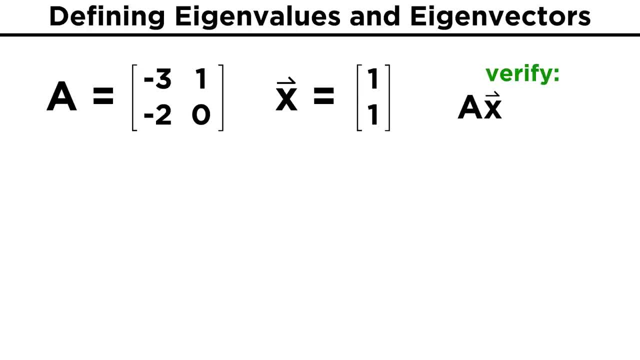 two and zero. To do this, we will simply multiply A by x and see if we get back x multiplied by some scalar. Performing the multiplication, we get negative three times one plus one times one. negative two times one plus zero times one, or negative three plus one. negative two plus zero. which? 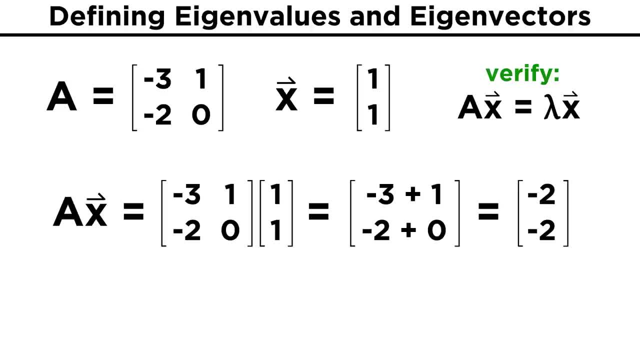 simplifies to negative two, negative two. We can simply factor out a negative two from this and get negative two times one, one which is just our original vector, multiplied by negative two. We have not only verified that one one is in fact an eigenvector of our matrix, but 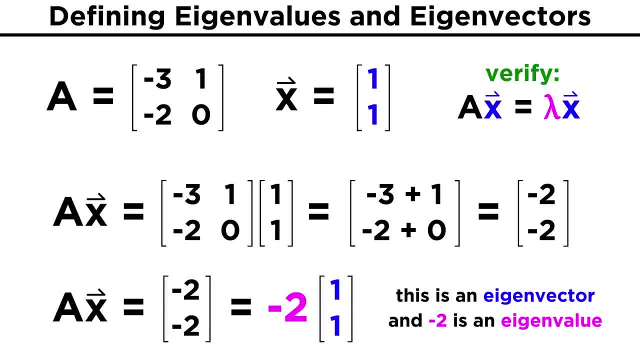 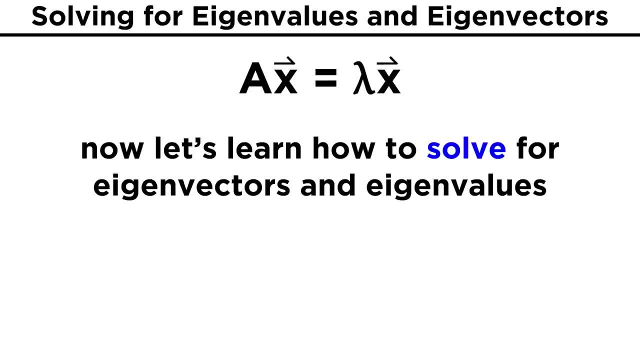 also discovered that negative two is one of its eigenvalues. Now that we are better acquainted with eigenvalues and eigenvectors, let's start learning how to solve for them. We know that the eigenvalues and eigenvectors of a square matrix A obey the equation Ax. 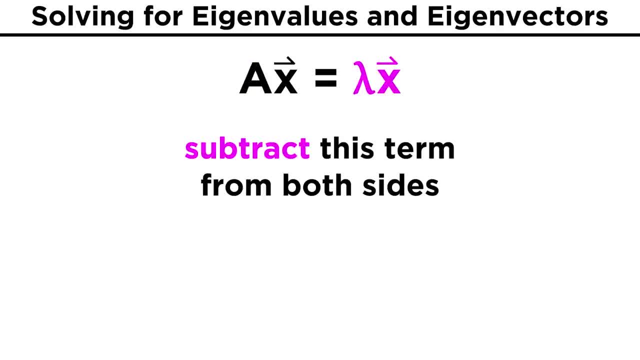 equals lambda x. In order to solve this, we will first subtract lambda x from both sides, Then, in between lambda and x, we will insert the identity matrix I, which is the matrix equivalent of multiplying by one. so we are not changing the equation by doing this. 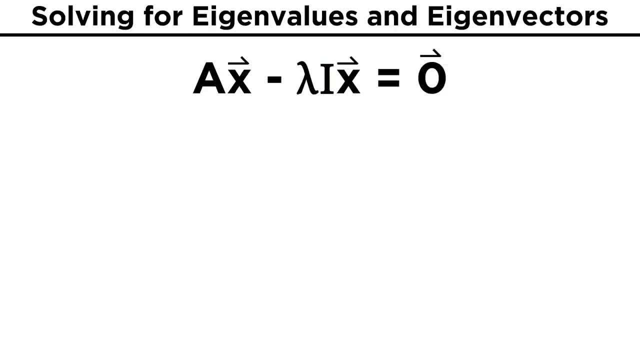 Okay, AX minus lambda IX equals the zero vector. If we factor out the vector, we can rewrite this as: the quantity A minus lambda I times X equals the zero vector. Now we want non-trivial solutions to this equation, meaning that X can't be the zero. 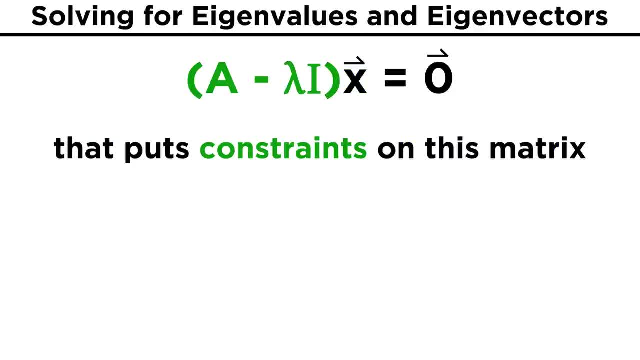 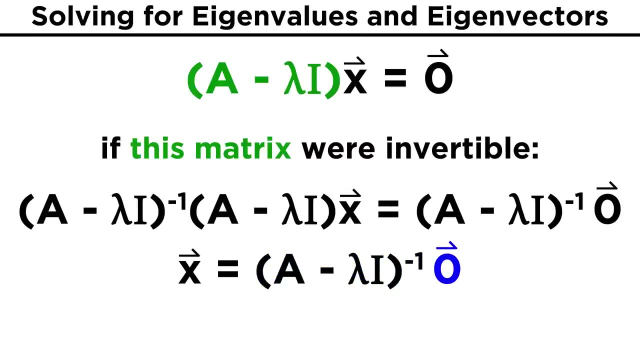 vector. Let's see what this means for A minus lambda I. If this matrix were invertible, then we could multiply both sides by A minus lambda I- inverse and get X equals A minus lambda I inverse times the zero vector, which would mean that 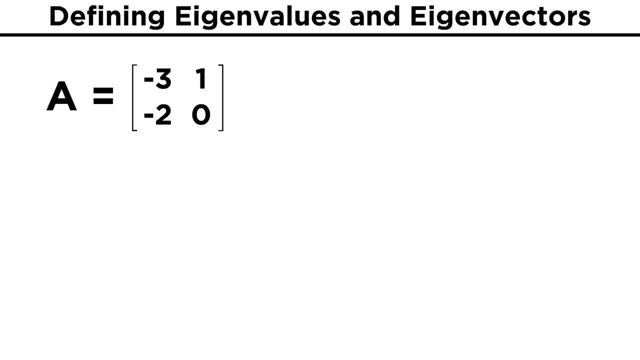 Let's say that matrix A is a two by two matrix with elements negative three, one negative two and zero. Now let's check that the vector x equals one. one is an eigenvector. Let's say that matrix A is a two by two matrix with elements negative three, one negative. 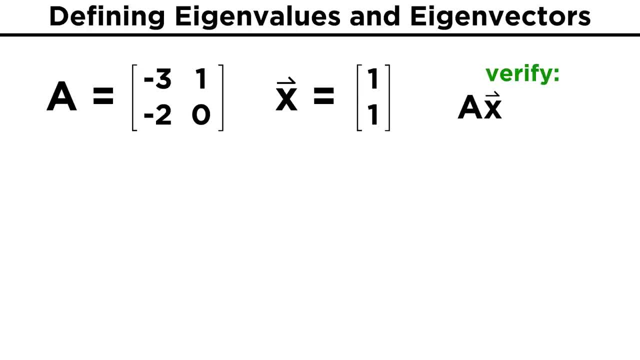 two and zero. To do this, we will simply multiply A by x and see if we get back x multiplied by some scalar. Performing the multiplication, we get negative three times one plus one times one. negative two times one plus zero times one, or negative three plus one. negative two plus zero. which? 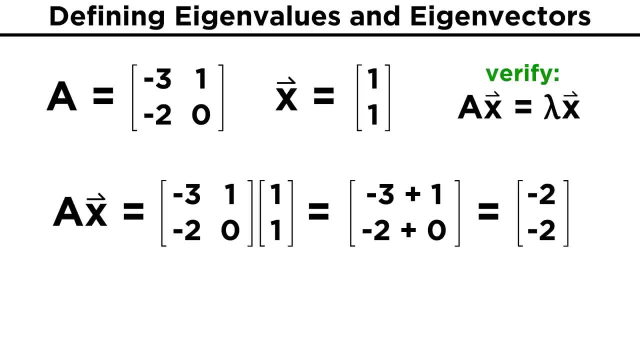 simplifies to negative two, negative two. We can simply factor out a negative two from this and get negative two times one, one which is just our original vector, multiplied by negative two. We have not only verified that one one is in fact an eigenvector of our matrix, but 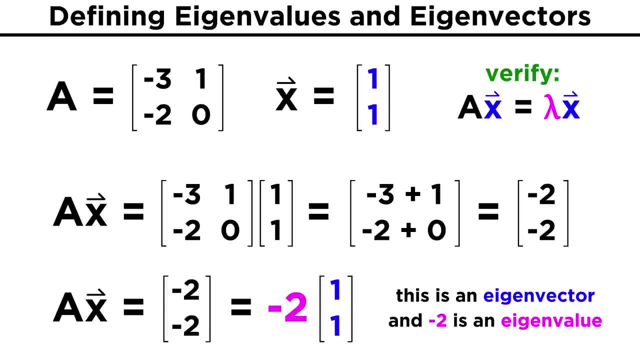 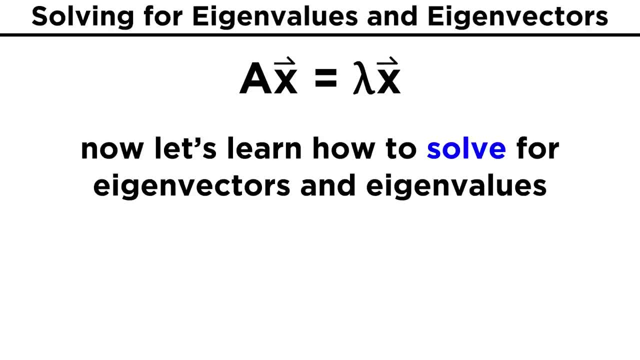 also discovered that negative two is one of its eigenvalues. Now that we are better acquainted with eigenvalues and eigenvectors, let's start learning how to solve for them. We know that the eigenvalues and eigenvectors of a square matrix A obey the equation AX equals. 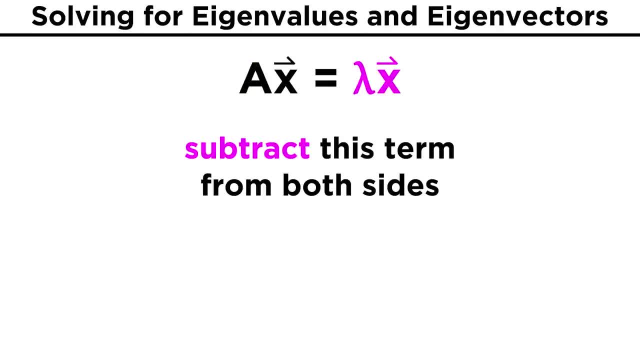 lambda x. In order to solve this, we will first subtract lambda x from both sides, Then in between lambda and x, we will insert the identity matrix I, which is the matrix equivalent of multiplying by one. so we are not changing the equation by doing this. 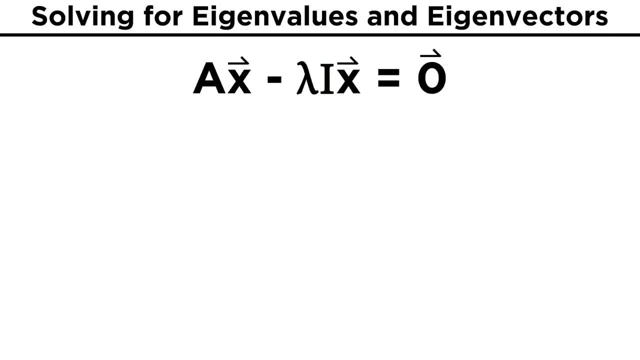 Now we have AX minus x. AX lambda, x minus lambda i, x equals the zero vector. If we factor out the vector, we can rewrite this as: the quantity A minus lambda i times x equals the zero vector. Now we want non-trivial solutions to this equation, meaning that x can't be the zero. 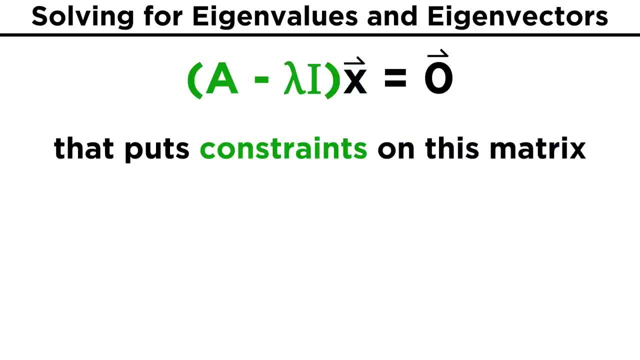 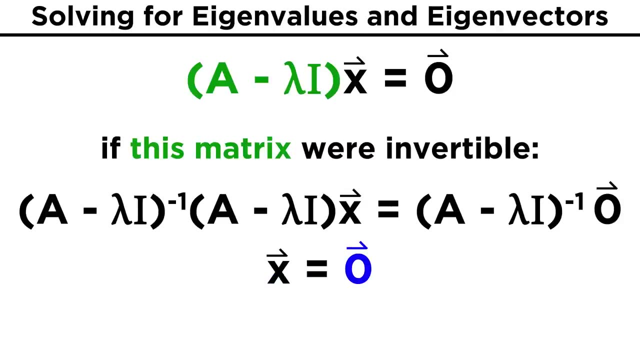 vector. Let's see what this means for A minus lambda i. If this matrix were invertible, then we could multiply both sides by A minus lambda i- inverse and get x equals A minus lambda i inverse times the zero vector, which would mean that 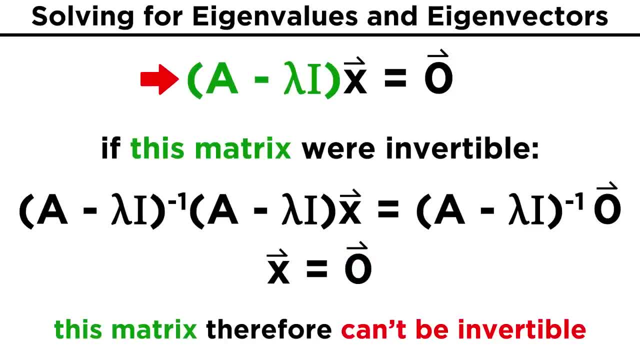 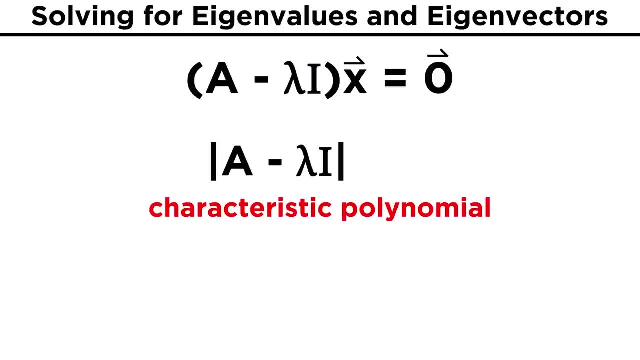 X is zero. To avoid this situation, A minus lambda I can't be invertible and therefore, as we recall from learning about inverse matrices, the determinant of this matrix must be zero, The determinant of A minus lambda I will form a polynomial in lambda, often referred. 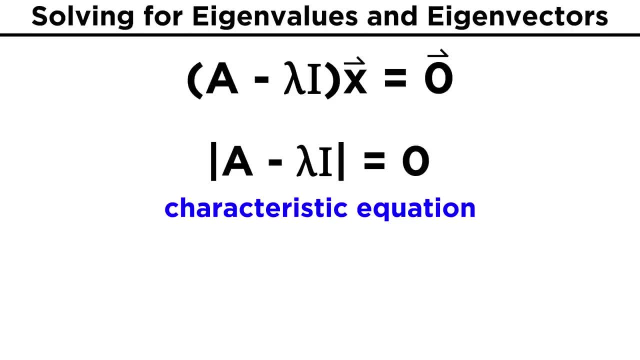 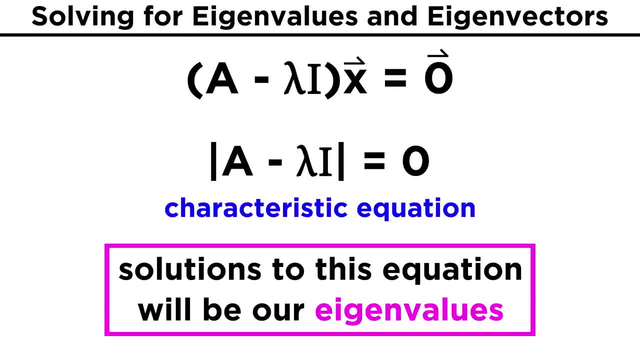 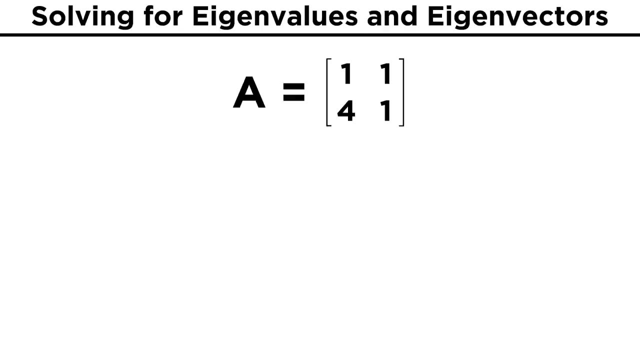 to as the characteristic polynomial, and the equation formed when the determinant equals zero is called the characteristic equation. The solutions to this equation will be our eigenvalues. Let's try a concrete example so that this will make more sense. Consider matrix A, which equals one. 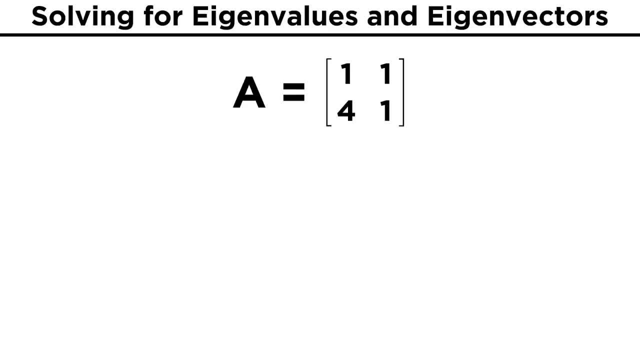 Let's try a concrete example so that this will make more sense. Consider matrix A, which equals one. It's one one four one. We will take this matrix and subtract lambda I, where I is, the two by two matrix with. 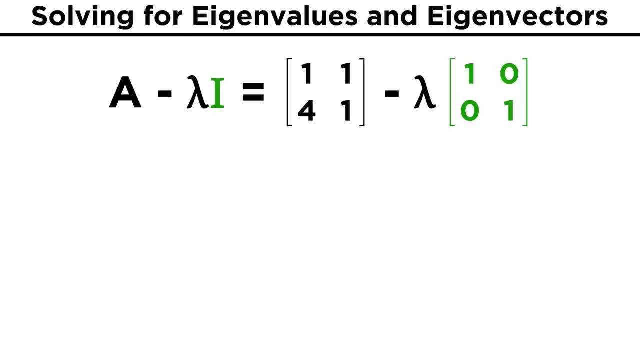 ones on the main diagonal and zeros for the other two entries. Multiplying by lambda, we simply end up with lambdas on the main diagonal, and so in performing the subtraction, we will simply end up subtracting lambda from the main diagonal of A. that gives 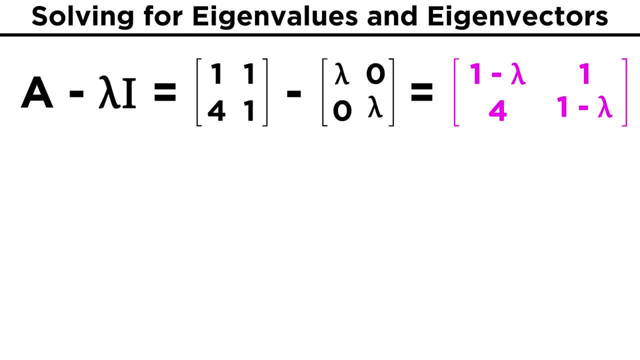 us one minus A minus lambda, I minus lambda, one four. one minus lambda. Now we must take the determinant of this matrix and set it equal to zero. The determinant will be one minus lambda times one minus lambda, minus the quantity four. 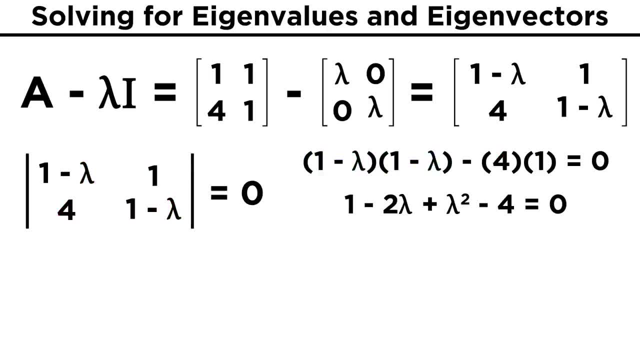 times one. Foiling out this first term leaves us with one minus two lambda plus lambda squared minus four. If we simplify and then set this equal to zero, that will give us a characteristic equation of lambda squared minus two. lambda minus three equals zero. 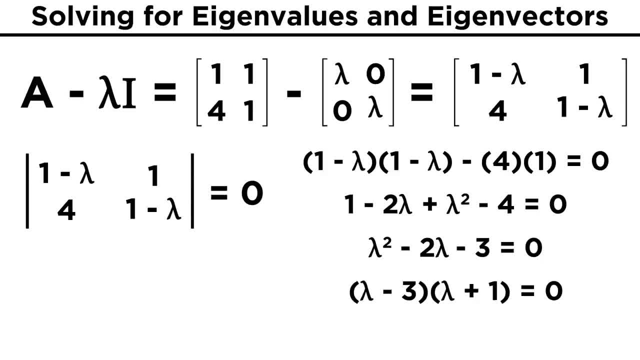 If we recall our basic algebra, we can easily factor this, rewriting it as: lambda minus three times lambda plus one equals zero. This means that we have two solutions, three and negative one. These are the eigenvalues. So to summarize what we just did, 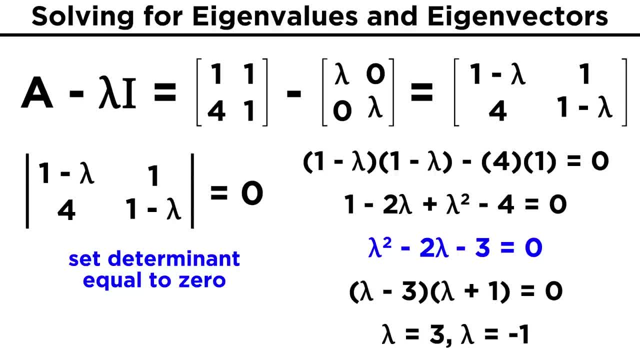 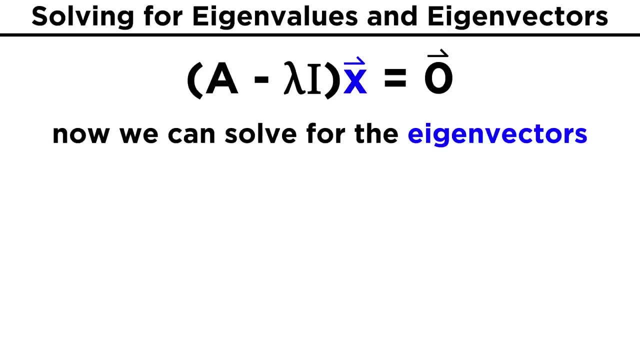 We found the determinant of A minus lambda I and set it equal to zero, which was our characteristic equation, and then solving that equation gave us a pair of eigenvalues. Once we have found the eigenvalues for a matrix, we can start solving for the eigenvectors. 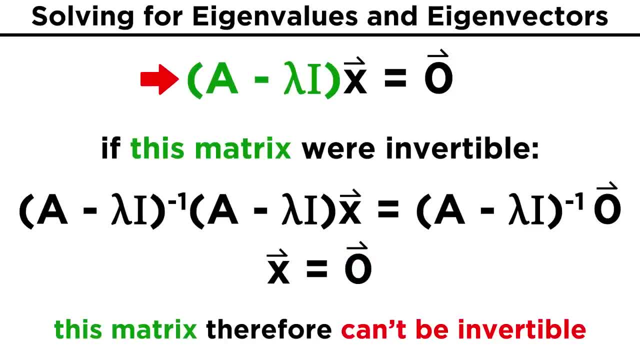 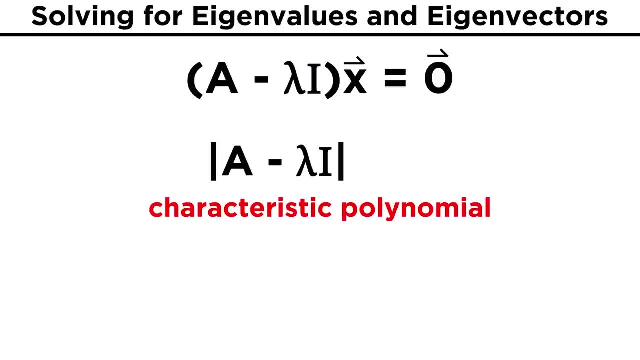 x is zero. To avoid this situation, A minus lambda i can't be invertible and therefore, as we recall from learning about inverse matrices, the determinant of this matrix must be zero. The determinant of A minus lambda i will form a polynomial in lambda, often referred. 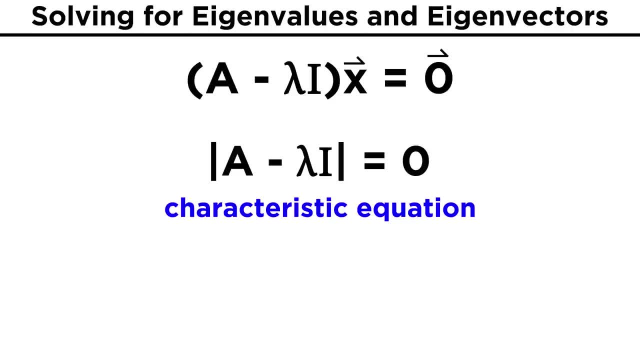 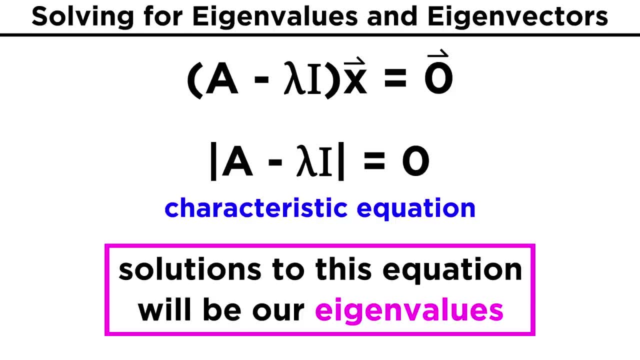 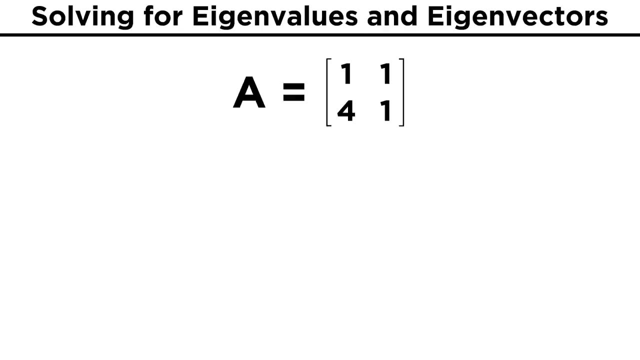 to as the characteristic polynomial, and the equation formed when the determinant equals zero is called the characteristic equation. The solutions to this equation will be our eigenvalues. Let's try a concrete example so that this will make more sense. Consider matrix A: one, one, four, one. 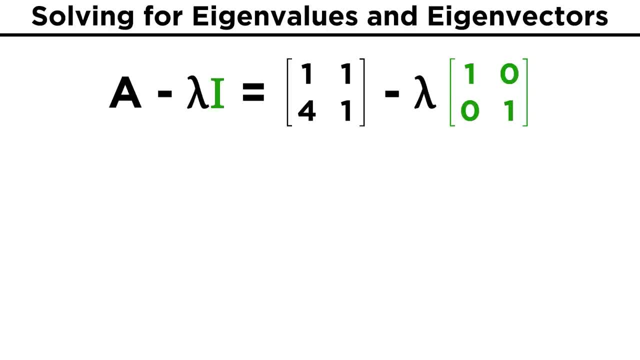 We will take this matrix and subtract lambda I, where I is the two by two matrix, with ones on the main diagonal and zeros for the other two entries Multiplying by lambda, we simply end up with lambdas on the main diagonal, and so in performing 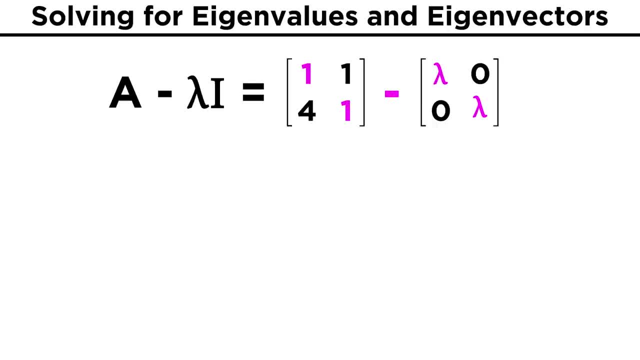 the subtraction. we will simply end up subtracting lambda from the main diagonal of A. That gives us one minus lambda, one four, one minus lambda. Now we must take the determinant of this matrix and set it equal to zero. The determinant will be one minus lambda times one minus lambda minus the quantity four. 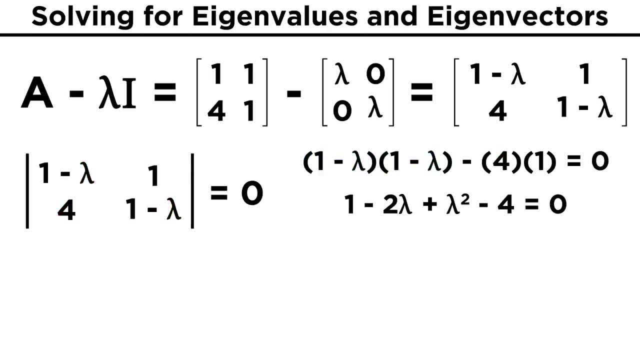 times one. Foiling out this first term leaves us with one minus two lambda plus lambda, squared minus four. If we simplify and then set this equal to zero, we get one minus lambda times one minus lambda. That's one minus lambda times one minus lambda. 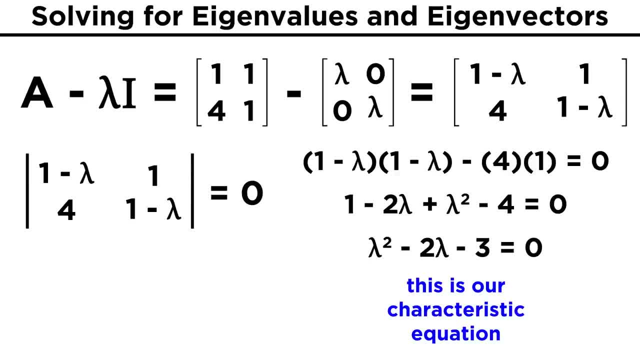 That will give us a characteristic equation of lambda squared minus two. lambda minus three equals zero. If we recall our basic algebra, we can easily factor this, rewriting it as: lambda minus three times lambda plus one equals zero. This means that we have two solutions: three and negative one. 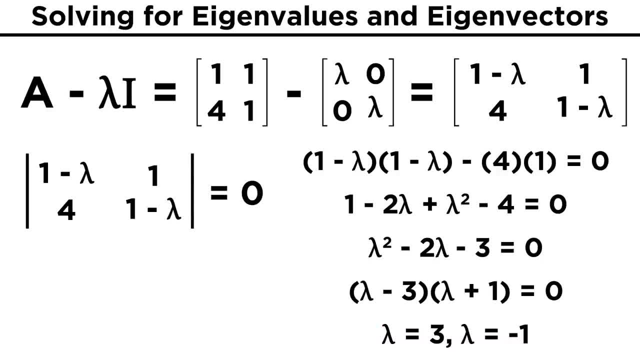 These are the eigenvalues. So, to summarize what we just did, we found the determinant of A minus lambda I equals one minus lambda I- and set it equal to zero, which was our characteristic equation. and then solving that equation gave us a pair of eigenvalues. 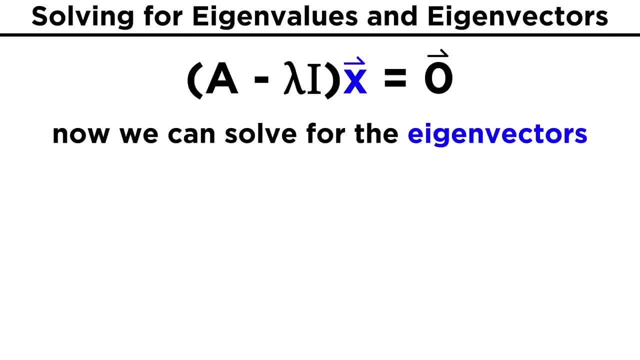 Once we have found the eigenvalues for a matrix, we can start solving for the eigenvectors. This takes a bit more effort and it must be done for each eigenvalue separately. We will once again start the process by examining the A minus lambda. I part of A minus lambda. 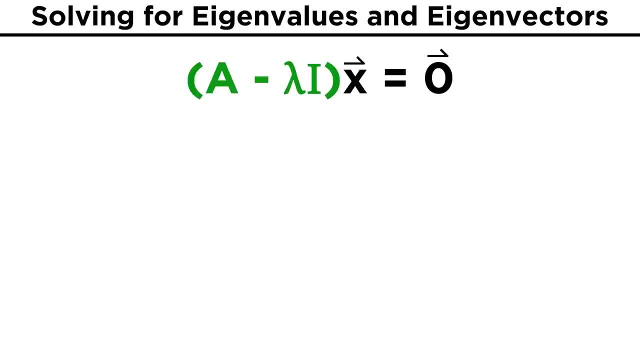 The A minus lambda- I part of A minus lambda I times X, equals the zero vector. This time we will actually plug in one of the eigenvalues we found for lambda and get a new matrix. This new matrix multiplied by our unknown vector, X equals zero. so in essence, what? 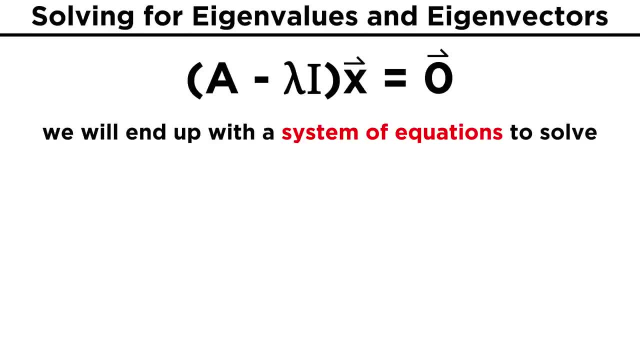 we are left with is a system of equations that we can solve by any method we've learned so far. The most consistent method here is to use row operations to get the matrix into row echelon form. There will be times when we must choose values for the components of the eigenvectors, but 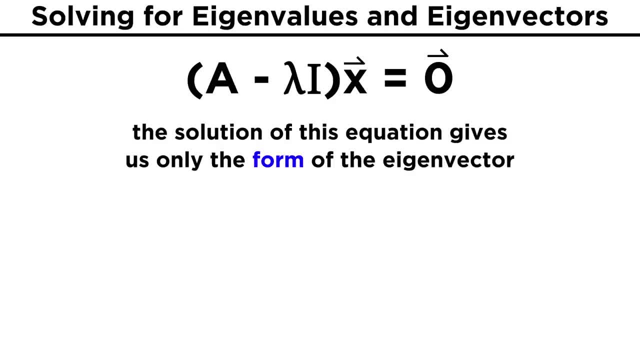 it doesn't really matter what we choose, because the solution we find by doing so only represents the form of eigenvectors. Any scalar multiple of the vector we find through this method will also be an eigenvector. We can easily demonstrate this as follows. 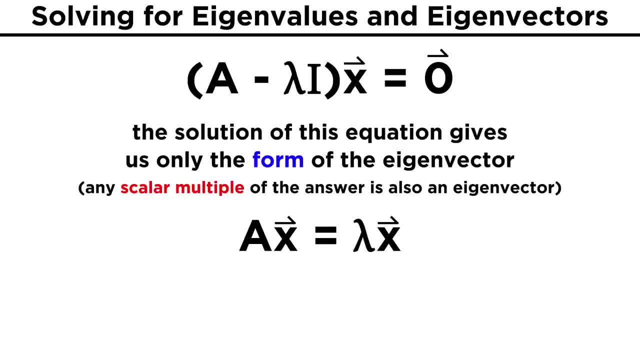 Assume the vector X is an eigenvector of X. We can easily demonstrate this as follows: Assume the vector X is an eigenvector of A, So AX equals lambda X. Now if we consider the vector CX, where C is a scalar, then A times this new vector. 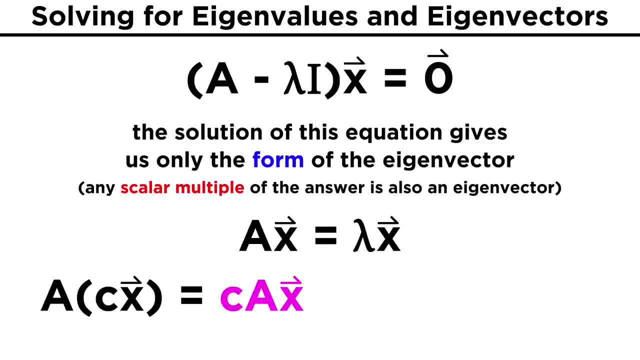 can also be written as C times AX, since C is just a scalar. We already know AX equals lambda X, so this becomes C lambda X, which can be rewritten as lambda CX. So we get A CX equals lambda CX, which makes the vector CX equal lambda CX, which is the 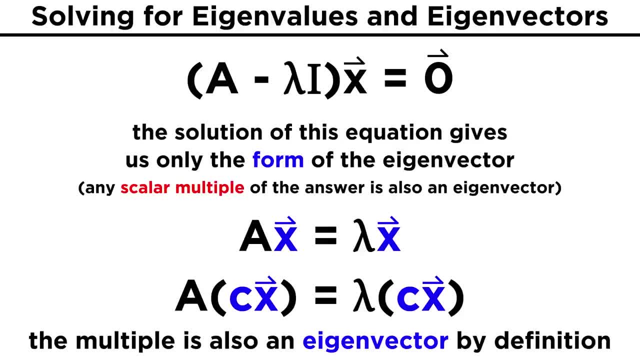 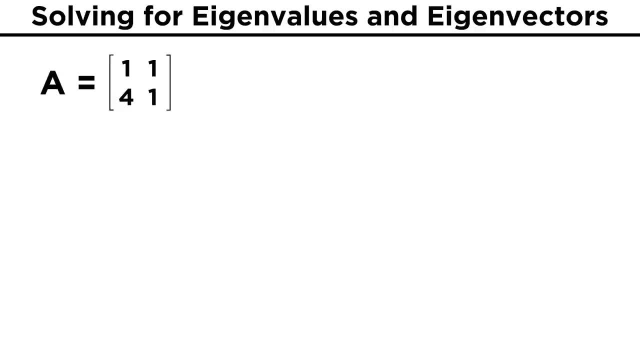 vector CX, an eigenvector by definition. To make this process of solving for eigenvectors a little more clear, let's once again consider the matrix A equals. We have already found the eigenvalues of this matrix to be three and negative one, so let's. 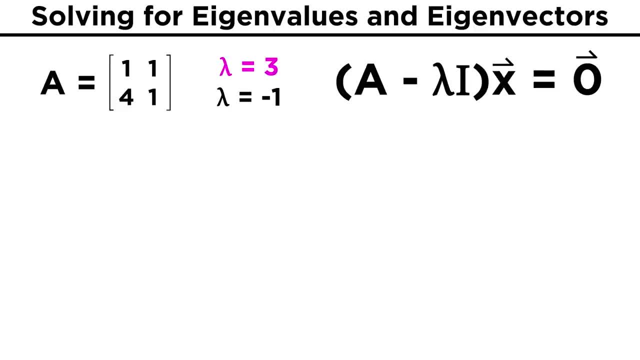 use these to find the related eigenvectors. We can start with lambda equals three and plug this into A minus lambda I, We end up getting threes on this main diagonal, which means we will be subtracting three from the diagonal elements of A, leaving us with negative two. one. four negative two. 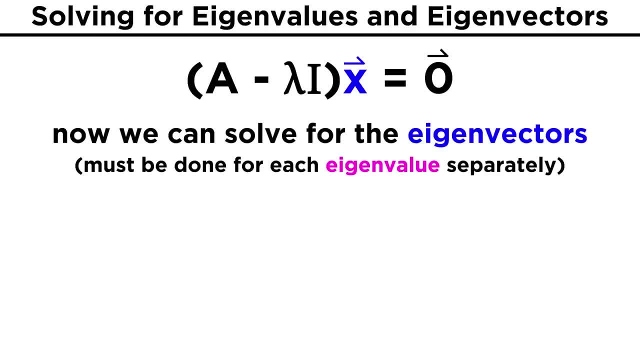 This takes a bit more effort and it must be done for each eigenvalue separately. We will once again start the process by examining the eigenvalues separately. We will once again start the process by examining the eigenvalues separately. This time we will actually plug in one of the eigenvalues we found for lambda and get. 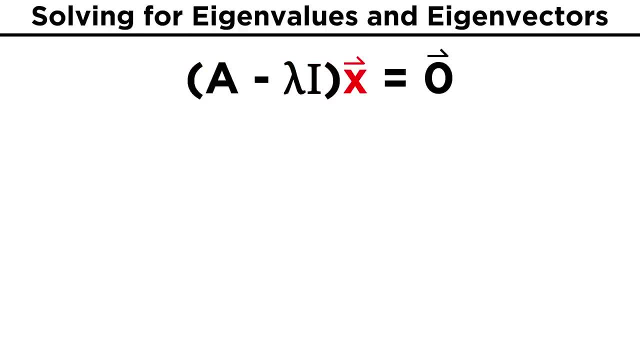 a new matrix. This new matrix, multiplied by our unknown vector x, equals zero. so, in essence, what we are left with is a system of equations that we can solve by any method we've learned so far. The most consistent method here is to use row operations to get the matrix equal to. 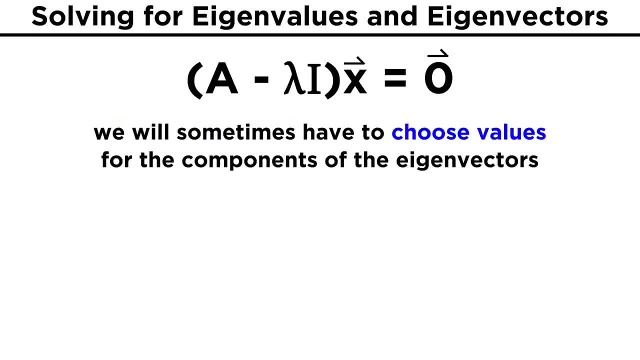 zero. We can use the matrix into row echelon form. There will be times when we must choose values for the components of the eigenvectors, but it doesn't really matter what we choose, because the solution we find by doing so only represents the form of eigenvectors. 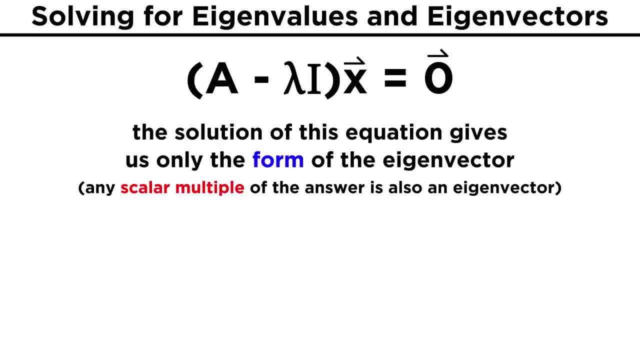 Any scalar multiple of the vector we find through this method will also be an eigenvector. We can easily demonstrate this as follows: Assume the vector x is an eigenvector of A, so A x equals lambda x. Now if we consider the vector C, x, where C is a scalar, then A times this new vector. 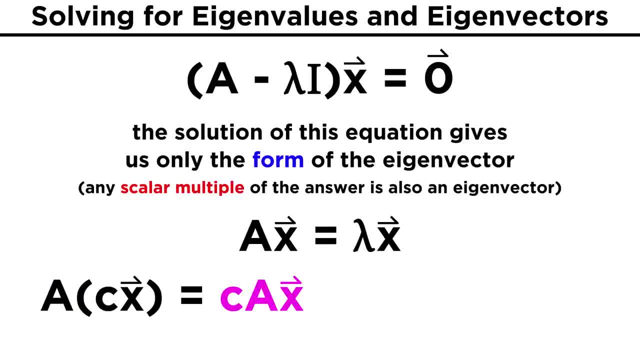 can also be written as C times A x, since C is just a scalar. We already know A x equals lambda x, so this becomes C lambda x, which can be rewritten as lambda C x. So we get A C x equals lambda C x, which makes the vector C x an eigenvector by definition. 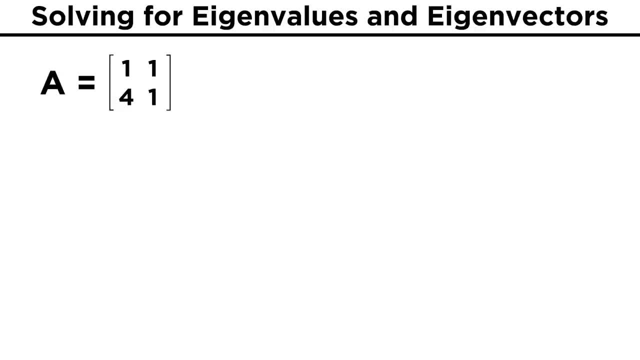 To make this process of solving for eigenvectors a little more clear, let's once again consider the matrix. A equals one, one four one. We have already found the eigenvalues of this matrix to be three and negative one, so let's use these to find the related eigenvectors. 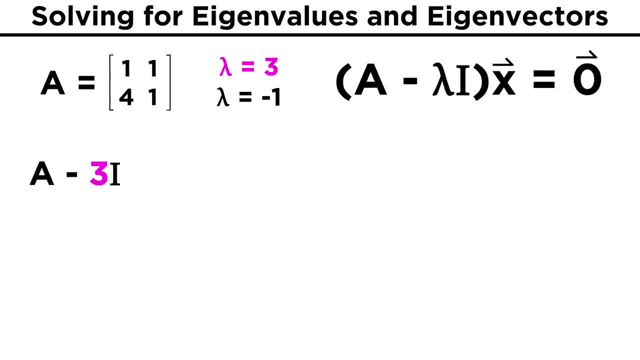 A equals three and plug this into A minus lambda I, We end up getting threes on this main diagonal, which means we will be subtracting three from the diagonal elements of A, leaving us with negative two, one, four negative two. 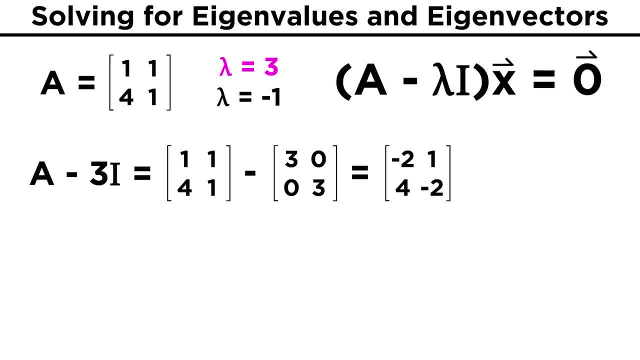 Now, once we have this, we will have to use row operations to get this in row echelon form. In this case, we can simply add two times the first row to the second row to get a new second row. This turns the second row into a new row. 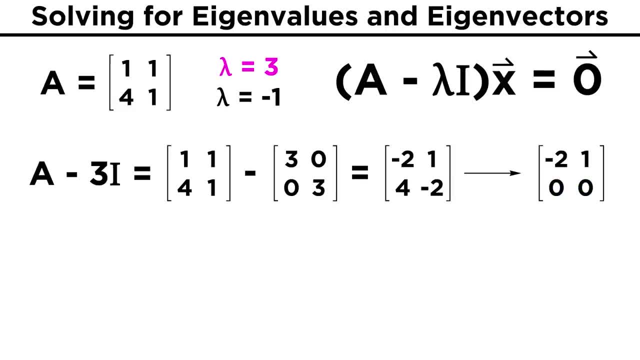 So we can simply add two times the first row to the second row to get a new second row. This turns the second row into a new row. So we can simply add two times the first row to get a new second row. This turns the second row into zeros and we are left with negative two and one in. 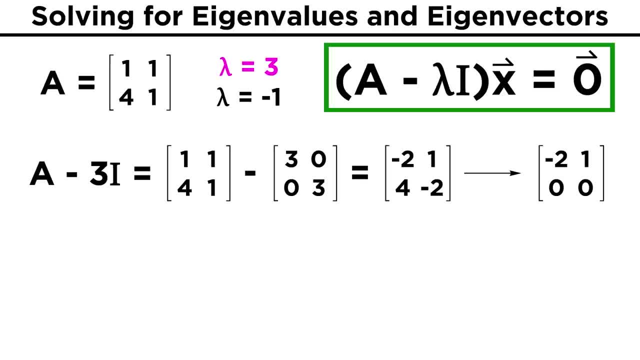 the first row. Recall that we are solving the matrix equation A minus lambda. i times x equals zero. so this matrix multiplied by x equals zero. Writing x as x1, x2, and doing matrix multiplication, we end up with the equation negative two x1. 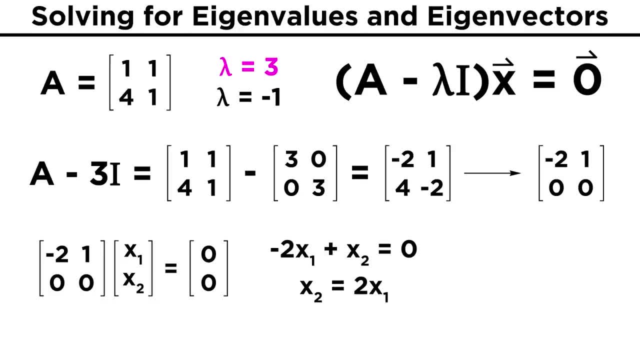 plus x2 equals zero. Moving two x1 to the other side, that leaves us with x2 equals zero. Next we add a new matrix to the real equation, adding X to the crazy math with a final. This gives us the following: 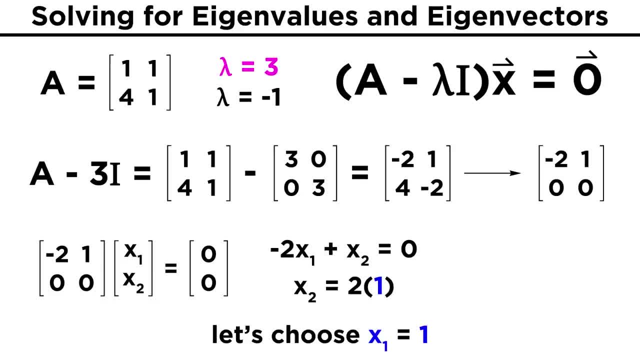 equals two x one. Let's now choose x one to be equal to one, which makes x two equal to two. So for the eigenvalue lambda equals three, we get the eigenvector x equals one- two. However, recall that this vector only represents the form eigenvectors. take for: 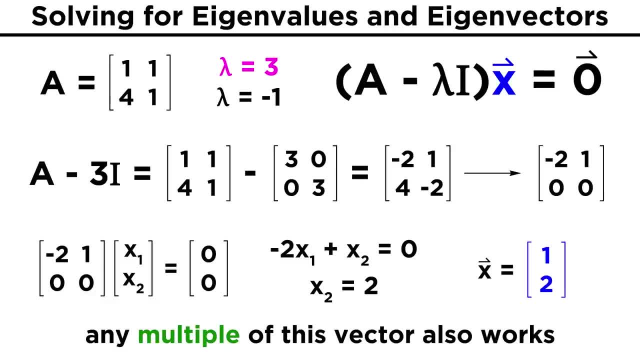 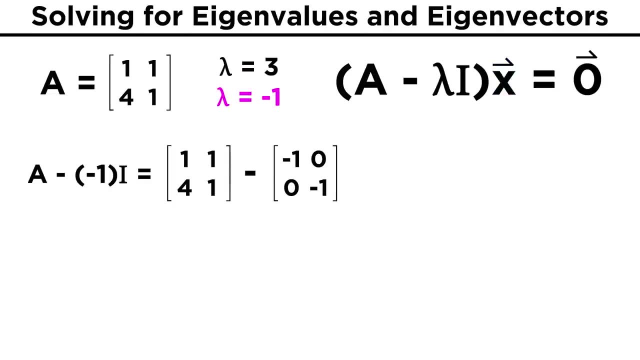 this eigenvalue. We can have any multiple of this vector and it will still be an eigenvector. To put it simply, any vector where the second element is twice the first will be an eigenvector. Now let's do the same thing for lambda equals negative one. We once again go back to A minus. 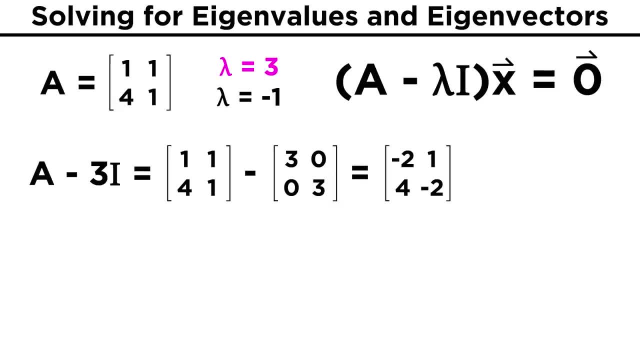 Now, once we have this, we will have to use row operations to get this in row echelon form. In this case, we can simply add two times the first row to the second row to get a new second row. This turns the second row into zeros and we are left with negative two and one in the 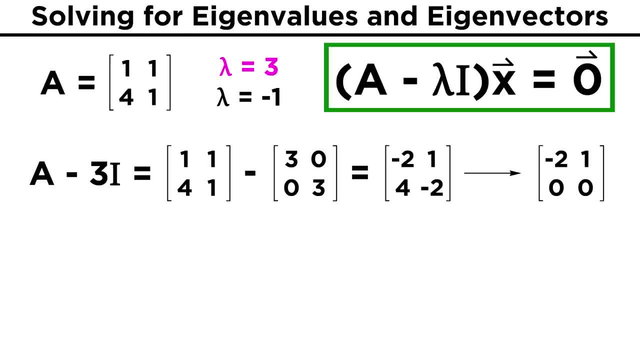 first row. Recall that we are solving the matrix equation. A minus lambda. I times X equals zero. so this matrix multiplied by X equals zero. Writing X as and doing matrix multiplication, we end up with the equation negative: two X one plus X two equals zero. 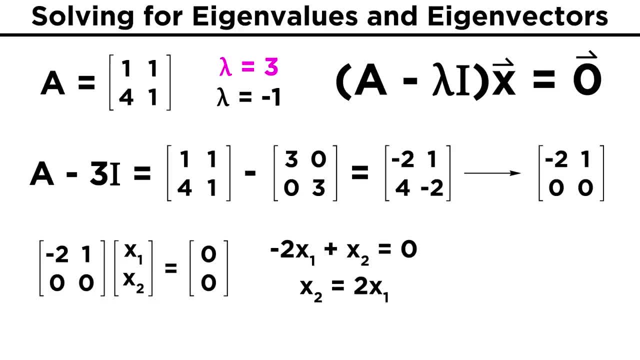 Moving two X one to the other side. that leaves us with X two equals two X one. Let's now choose the matrix equation. We can now choose X one to be equal to one, which makes X two equal to two. So for the eigenvalue lambda equals three, we get the eigenvector X equals one, two. 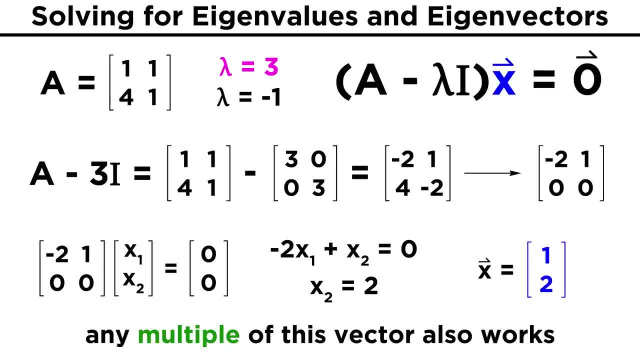 However, recall that this vector only represents the form eigenvectors take for this eigenvalue. We can have any multiple of this vector and it will still be an eigenvector. To put it simply, any vector where the second element is twice the first will be an eigenvector. 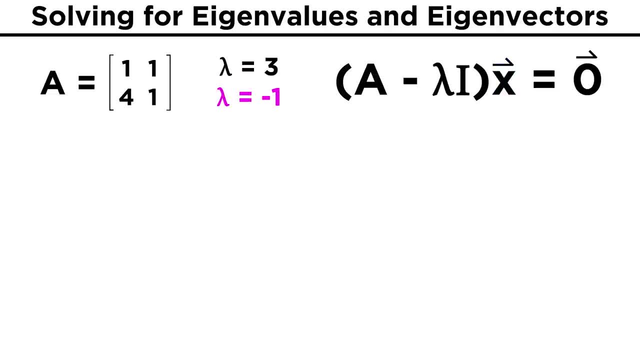 Thank you. Now let's do the same thing for lambda. equals negative one. We once again go back to A minus lambda, I, this time plugging in negative one for lambda. In this case, by subtracting negative one from the main diagonal of A, we find the result. 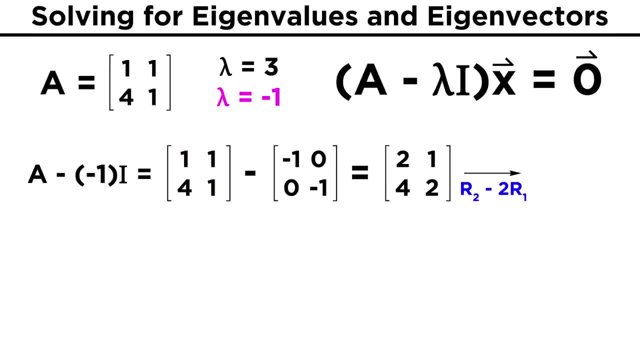 to be two, one, four, two For our row operation. this time we will subtract two times the first row from the second row to get a new second row. We are left with two and one in the first row. We are left with two and one in the second row, which this time makes our equation two. 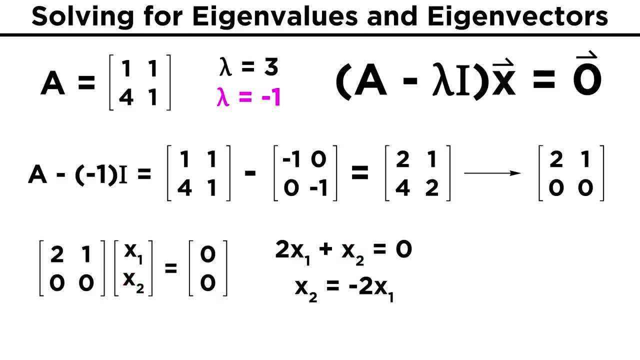 X one plus X two equals zero. Moving X one to the other side, we are left with X two equals negative two X one. Keeping it simple, let's again choose one for X one and we get X two equals negative two. making our vector: X equals one, negative two. 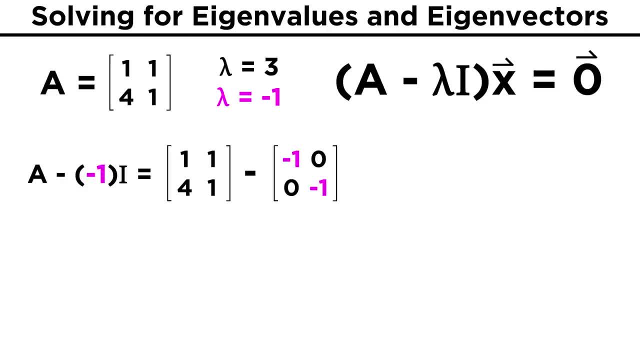 lambda I, this time plugging in negative one for lambda. In this case, by subtracting negative one from the main diagonal of A, we find the result to be two. one four two For our row operation. this time we will subtract two times the number of the first element. 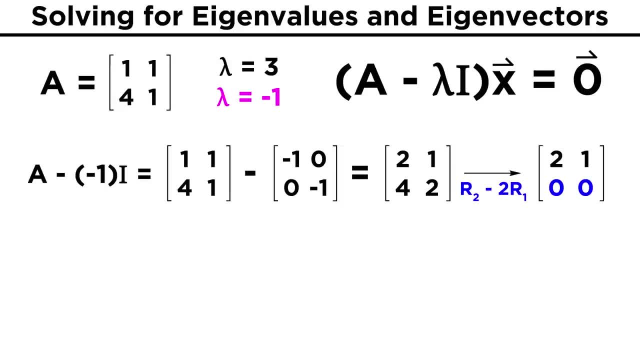 times the first row. from the second row to get a new second row, We are left with two and one in the first row, which this time makes our equation two x one plus x two equals zero. Moving x one to the other side, we are left with x. two equals negative two x one. 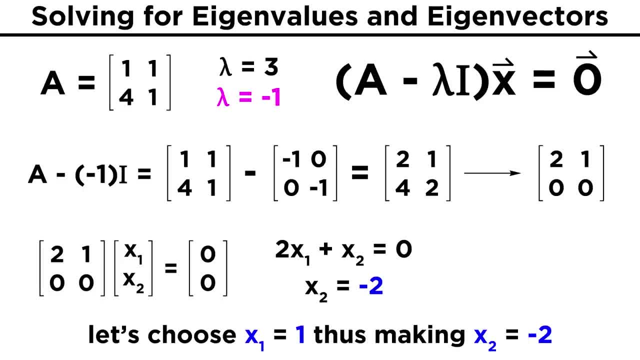 Keeping it simple, let's again choose one for x one and we get x two equals negative two, making our vector x equals one, negative two. Again, any multiple of this vector will also qualify. So the eigenvectors for lambda- equals negative one are vectors with their second element. 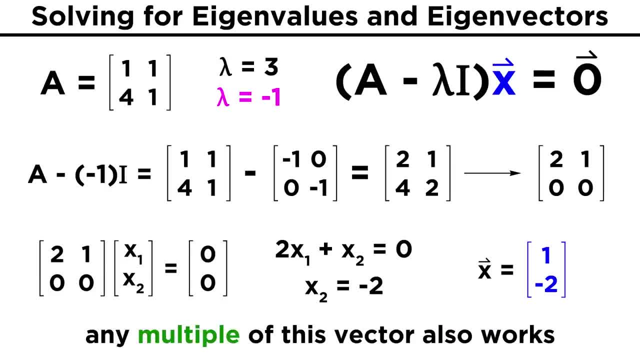 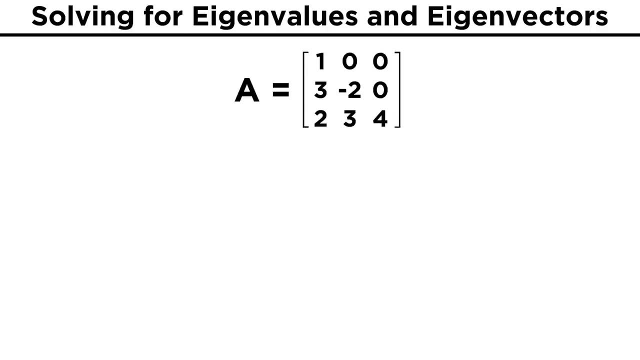 Again, any multiple of this vector will also qualify. So the eigenvectors for lambda equals negative one are vectors with their second element being equal to negative two times the first element. Now that we've gotten our feet wet, let's go through one more example to really make. 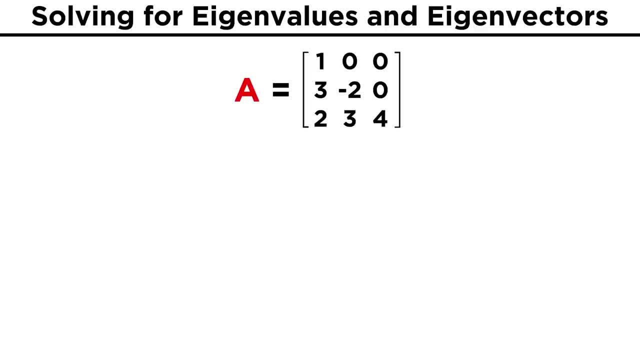 sure we understand this process. This time let's take our matrix A, to be one zero, zero, three, negative, two zero, two, three, four, and for this we will find the eigenvalues and eigenvectors. First to find the eigenvalues, let's find A minus lambda I, which will mean subtracting. 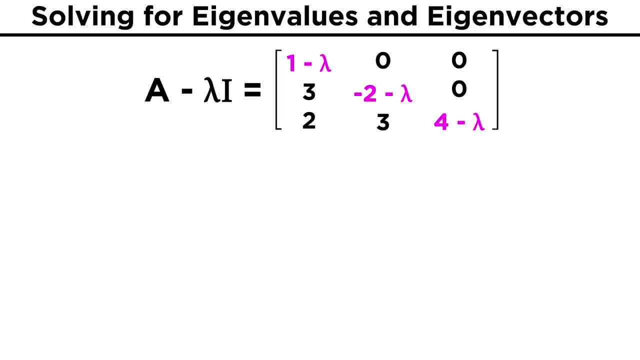 lambda from the second element. Then we will take the determinant of this new matrix and set the polynomial equal to zero. Thanks to the form of our matrix, with two zeros in the top row, the determinant of A minus lambda I is relatively simple. 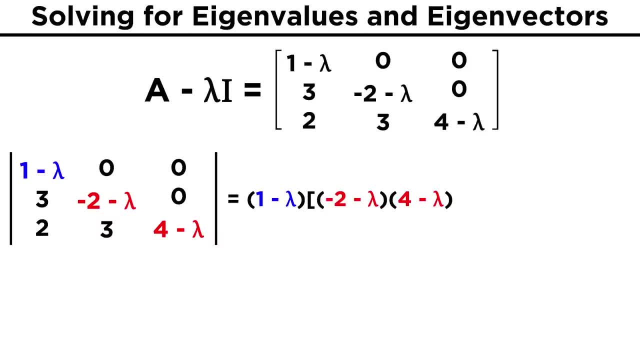 We get one minus lambda times negative, two minus lambda times four minus lambda minus zero times three, then minus zero and then plus zero. This simplifies to the product of these three binomials, and setting this equal to zero, we end up with a characteristic equation that is already completely factored. 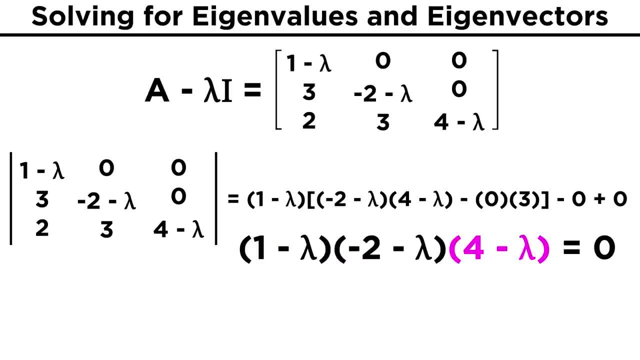 One minus lambda times negative, two minus lambda times four minus lambda equals zero. So our solutions are: lambda equals one, lambda equals negative two and lambda equals four. and these are the eigenvalues for this matrix. Now that we have the eigenvalues, let's go ahead and find the eigenvalues for lambda. 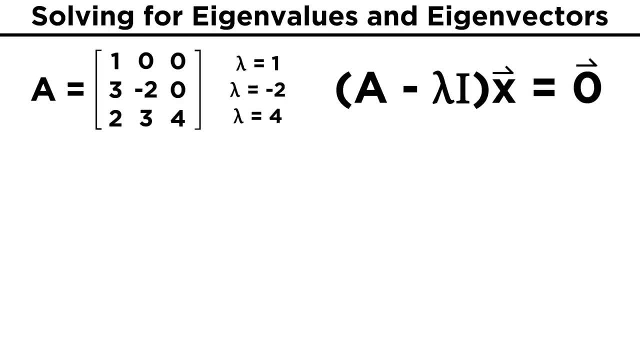 Let's do that. If we have the eigenvalues, we can solve for the eigenvectors that are related to each of them. Let's start with lambda equals one. We will go back to our matrix given by A minus lambda I and plugging in lambda equals one. 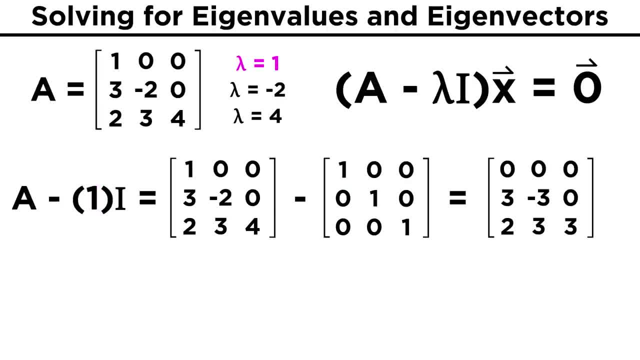 we will subtract one from the terms in the main diagonal to get the matrix zero, zero, zero, three. negative, three, zero, two, three, three. We could go through row operations from here, but the form of our matrix in this case may make it simple to solve if we jump right into equation form. 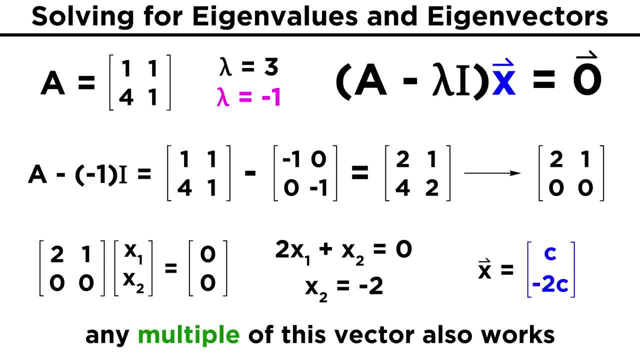 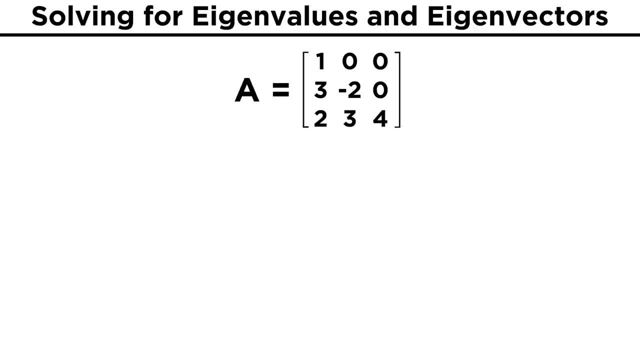 being equal to negative two times the first element. Now that we've gotten our feet wet, let's go through one more example to really make sure we understand this process. This time let's take our matrix A to be one zero zero. three negative two zero two. 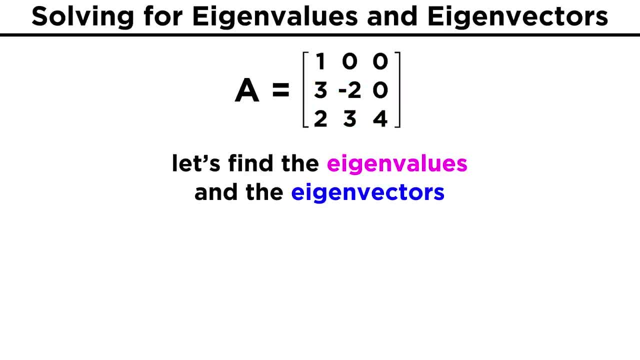 three, four, and for this we will find the eigenvalue and eigenvectors. First to find the eigenvalues, let's find A minus lambda I, which will mean subtracting lambda from the terms in the main diagonal of A. Then we will take the determinant of. 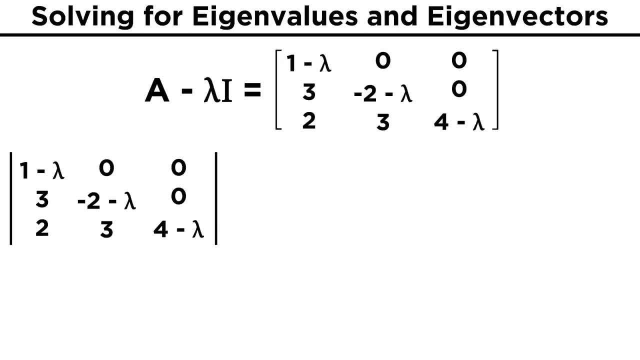 this new matrix and set the polynomial equal to zero. Thanks to the form of our matrix, with two zeros in the top row, the determinant of A minus lambda I is relatively simple. We get one minus lambda times negative, two, Two minus lambda times four, minus lambda minus zero times three, then minus zero, and. 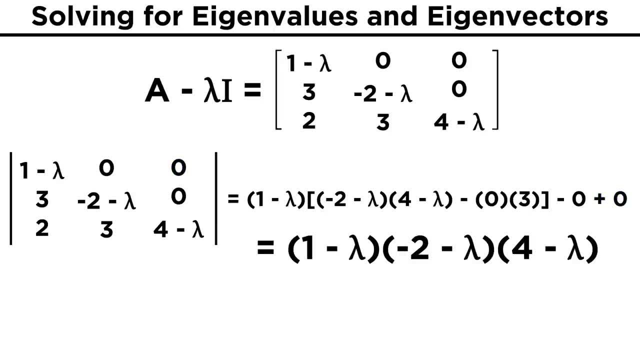 then plus zero. This simplifies to the product of these three binomials, and setting this equal to zero, we end up with a characteristic equation that is already completely factored: One minus lambda times negative. two minus lambda times four minus lambda equals zero. 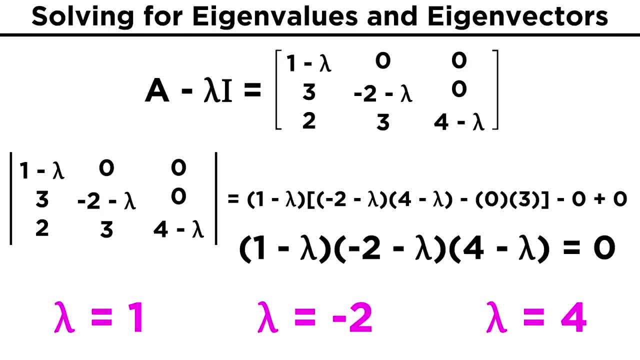 So our solutions are: lambda equals one, Lambda equals negative two And lambda equals four. And these are the eigenvalues for this matrix. Now that we have the eigenvalues, we can solve for the eigenvectors that are related to each of them. 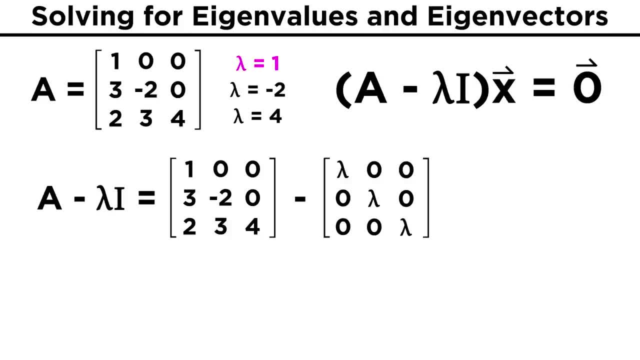 Let's start with lambda equals one. We will go back to our matrix given by A minus lambda I and plugging in lambda equals one. we will subtract one from the terms in the main diagonal to get the matrix zero, zero, zero, Three. negative three, zero, two, three, three. 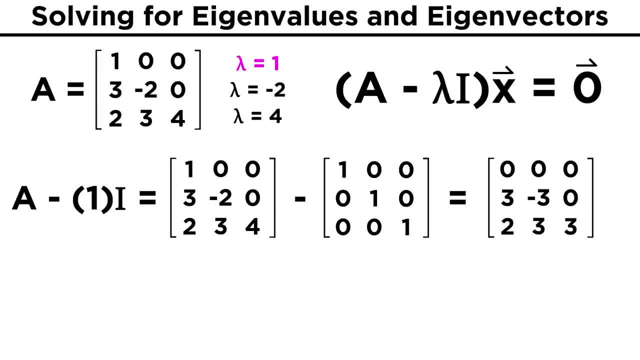 We could go through row operations from here, but the form of our matrix in this case makes it simple to solve. if we jump right into equation form, The top row gives no information, but the second row tells us three X one minus three X two equals zero. 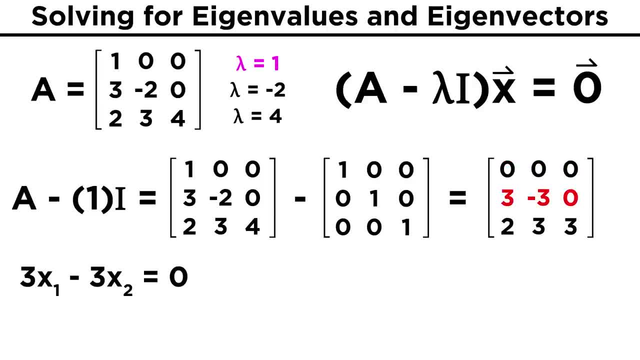 The top row gives no information, but the second row tells us: three X one minus three X two equals zero. Solving this, we see that X one equals X two and for this case let's choose X two to be one. So both X one and X two are therefore equal to one. 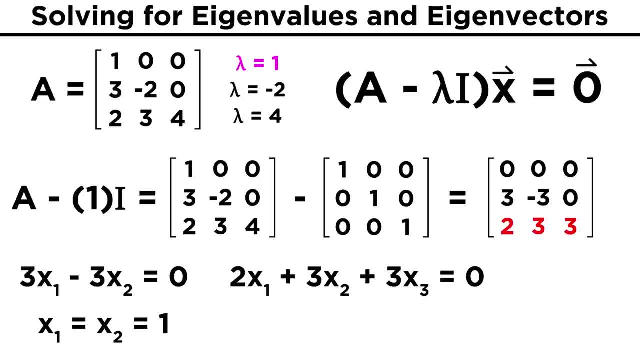 The final row tells us that two X one plus three, X two plus three X three equals zero. but we've already chosen X one plus three X three equals zero, so we can't solve for that. The final row tells us that X one and X two to be equal to one, so plugging those values. 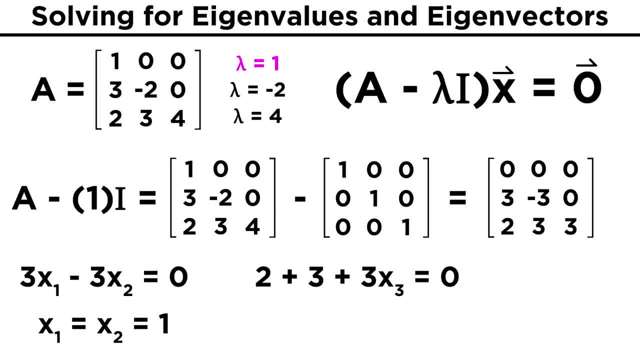 in. we get two plus three plus three. X three equals zero. We end up getting X three equals negative five thirds, making our eigenvectors any multiple of one one negative five thirds. Next we will find the eigenvectors for lambda equals negative two. 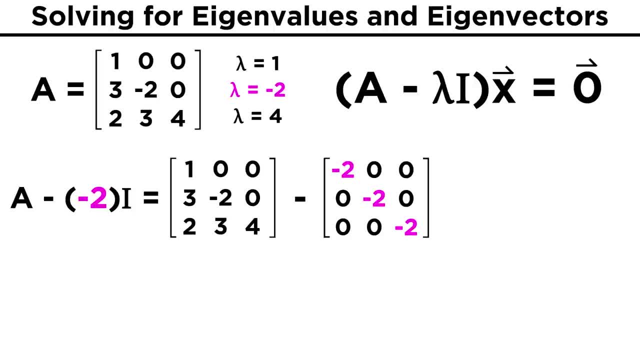 Plugging this value into A minus lambda I. we subtract negative two from the main diagonal to get three zero zero. We get three zero zero. three zero zero, two, three, six. Expressing this in equation form, the first row tells us that three X one equals zero. 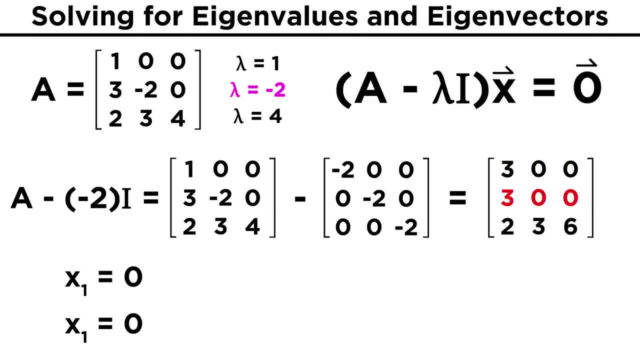 so X one must be zero. The second row tells us the same thing. Meanwhile, the final row becomes: two X one plus three X two plus six X three equals zero. We already know that X one is zero, so we are left with three X two plus six X three. 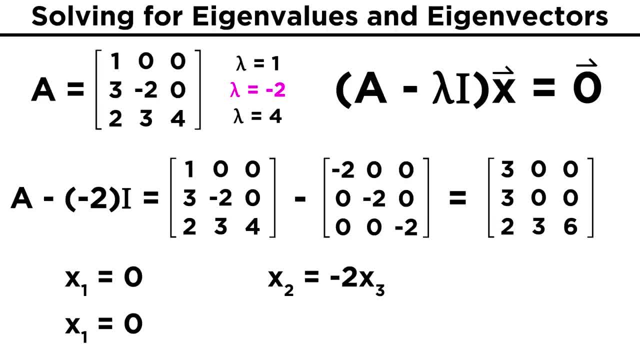 equals zero. We will now choose X three to be one, making X two equal to negative two. so the eigenvectors have the form zero, negative two, one. And finally, let's do the third eigenvalue: lambda equals four. 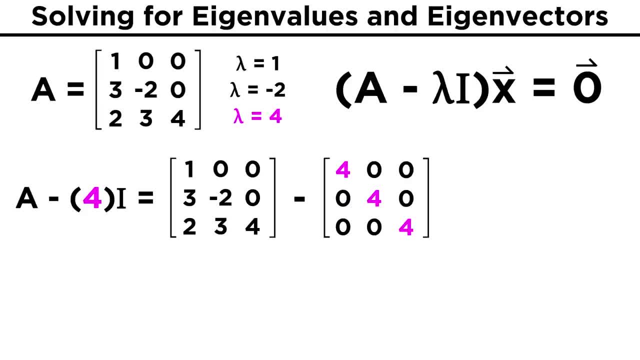 The matrix A minus lambda, I requires subtracting four from the main diagonal, so this becomes negative. three zero, zero. Three negative six equals zero. Three negative six equals zero. Three negative six equals zero. two, three, zero. The first row tells us that negative three X one equals zero. so once again, X one is. 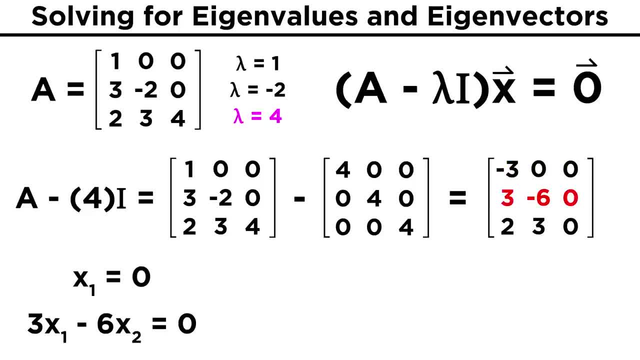 zero. The second row tells us three X one minus six X two equals zero. but since X one is zero, we are left with negative. six X two equals zero, so X two must also be zero. The third row becomes: two X one plus three X two equals zero. 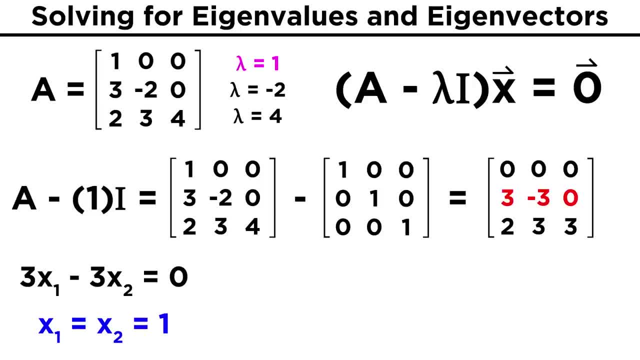 Solving this, we see that X one equals X two, and for this case let's choose X two to be one, So both X one and X two are therefore equal to one. The final row tells us that two X one plus three X two plus three X three equals zero. 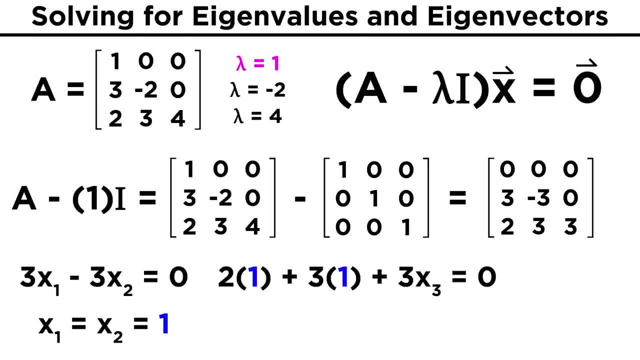 But we've already chosen X one and X two to be equal to one. So plugging those values in, we get two plus three plus three. X three equals zero. We end up getting X three equals negative five thirds, making our eigenvectors any multiple. 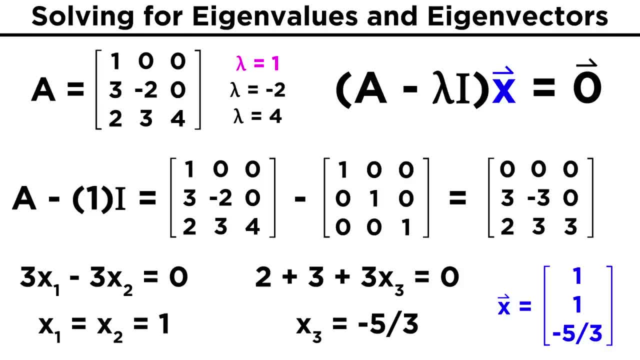 of one one negative five thirds. Next, we will find the eigenvectors for lambda equals one. We will go back to our matrix given by A minus lambda I. and we will go back to our matrix given by lambda equals negative two, Plugging this value into A minus lambda I. we subtract negative two from the main diagonal. 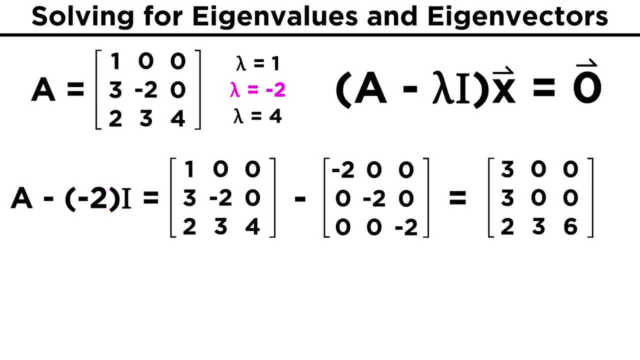 to get three zero zero. three zero zero two, three, six. Expressing this in equation form, the first row tells us that three X one equals zero, so X one must be zero. The second row tells us the same thing. Meanwhile, the final row becomes two X one plus three X two plus six X three equals zero. 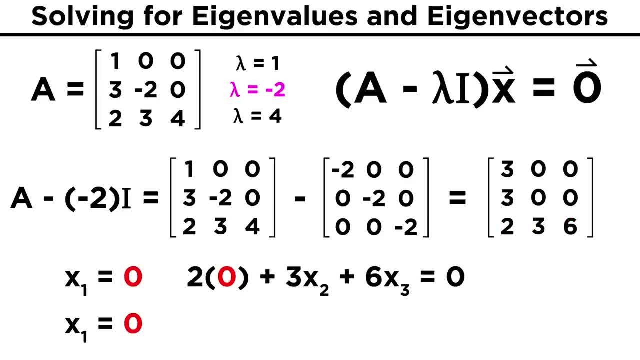 We already know that X one is zero, so we are left with three X two plus six. X three equals zero or X two equals negative. two X three. We will now choose X three to be one, making X two equal to negative two. 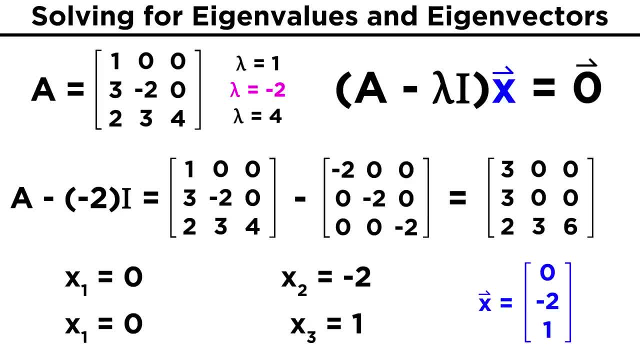 So the eigenvectors have the form zero, negative, two, one. And finally let's do the third eigenvalue: lambda equals four, The matrix A minus lambda. I requires subtracting four from the main diagonal, so this becomes negative. three, zero, zero, three negative six, zero, two, three, zero. 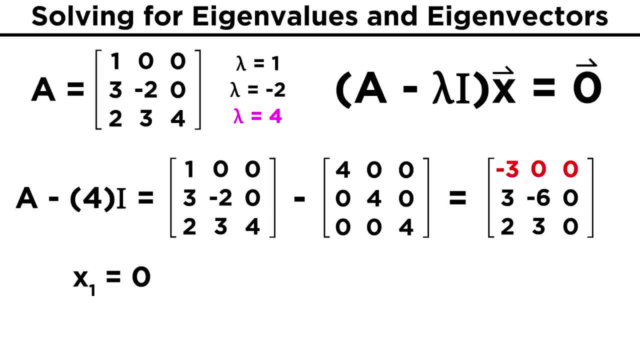 The first row tells us that negative three X one equals zero, so once again, X one is zero. The second row tells us: three X one minus six X two equals zero. but since X one is zero, we are left with negative. six X two equals zero.